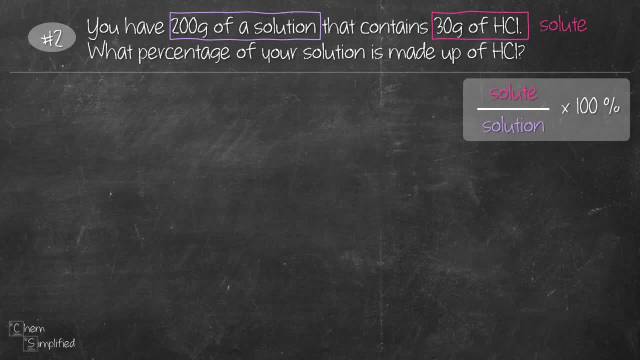 you think is the solute here? Yep, it's the HCl. So we'll place the solute on top, which is the 30 grams of HCl divided by the solution, which is 200 grams times 100%, And that works out to be 15%, Since. 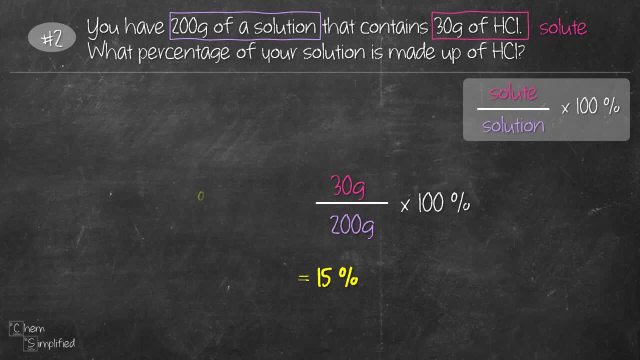 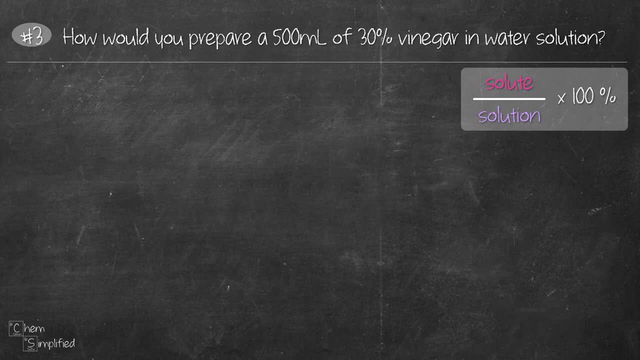 it's mass over mass, that 15% is the percent mass, which is abbreviated as percent m over m. Are you feeling good about this? Now we move on to a slightly harder question. Notice now: instead of given the solute and solution, we now have the percentage. instead, We're given the. 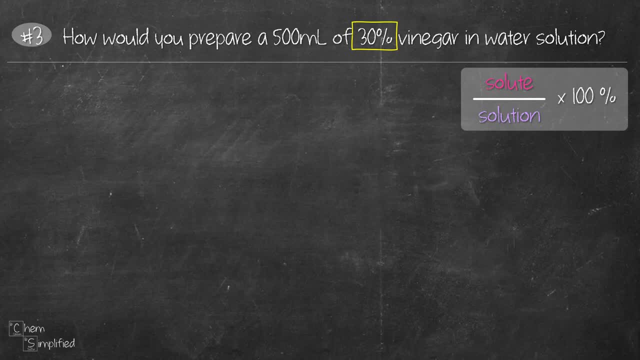 percent concentration for vinegar in water solution. You see how it's worded: Vinegar in water solution. That means vinegar is the solute and water is the solvent. The reason being solute is always dissolved in the solvent, So together solute and solvent. 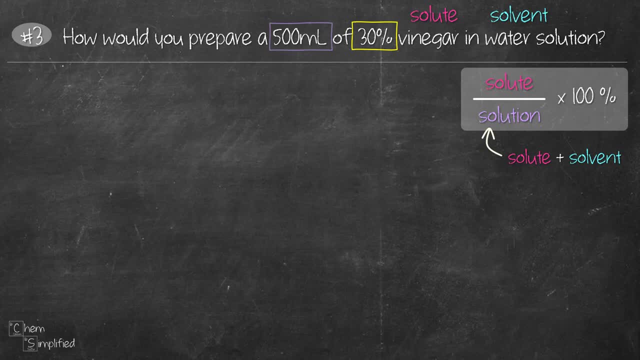 will mix to become the solution. The other piece of information we have is the 500 mL. Read the question carefully and you'll notice that the 500 mL is referring to the solution. So, to answer the question, we need to explain how to prepare this solution. 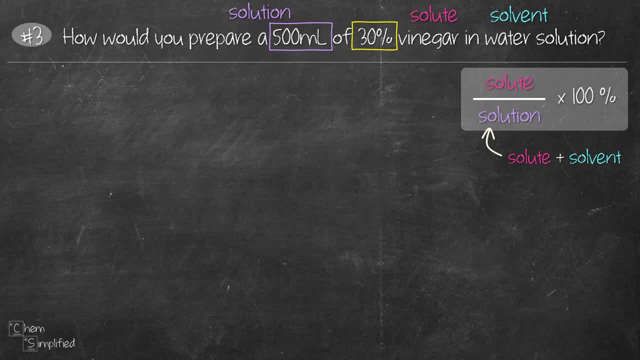 That means we need to figure out how much solute and solvent we need. So we know that vinegar and water are both in liquid form. That means the 30% is the percent volume, So 30% equals volume, meaning that 30% is the difference between itsnar and 30%, So 30% equals volume. 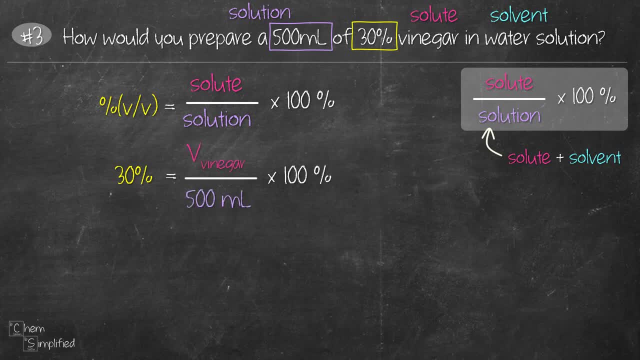 of vinegar which we do not have, divided by 500 ml times 100. We need to solve for the volume of vinegar. so we need to do a little bit of algebra. If we multiply with 500 and divide by 100, we can solve for the volume of vinegar. Since we did that on the right hand side, we need to do the same thing. 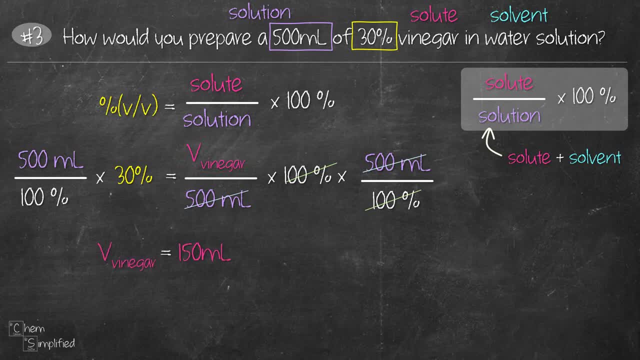 on the left hand side. So the volume of vinegar works out to be 150 ml, which came from 500 divided by 100 times 30. Since the solution is made out of vinegar and water, we can find a volume of water by subtracting the volume of vinegar from the solution, and that works out to be 350 ml. 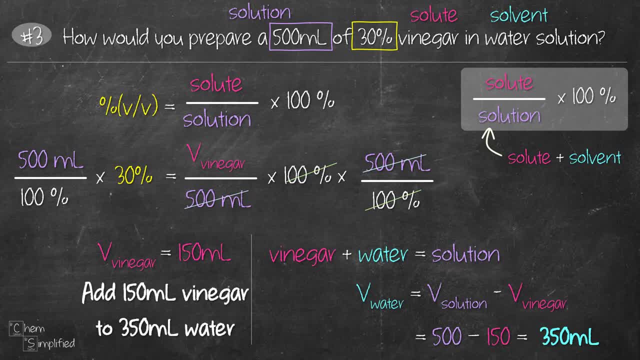 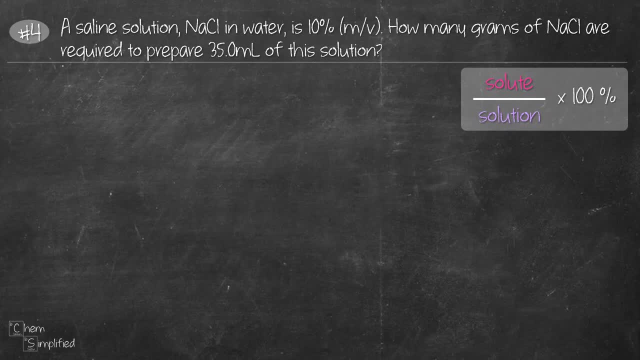 So to prepare the 30% vinegar in water solution, we need to add 150 ml of vinegar to 350 ml of water. Now notice this question: we have NaCl in water, Which is the solute and which is the solvent. Yeah, you got it.